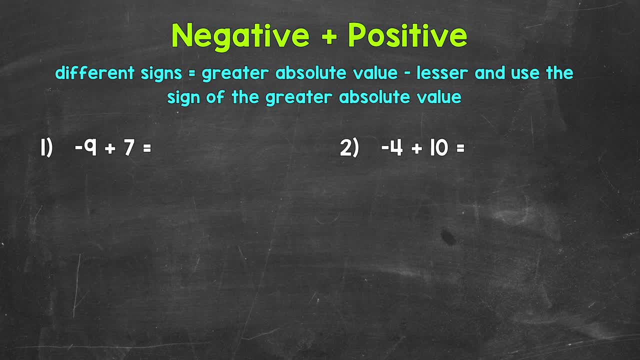 examples. Let's jump into number one, where we have negative nine plus seven. The first thing that we need to do is look at the signs For number one. we have a negative nine and a positive seven, So we have different signs: A negative and a positive. Since we have different signs, 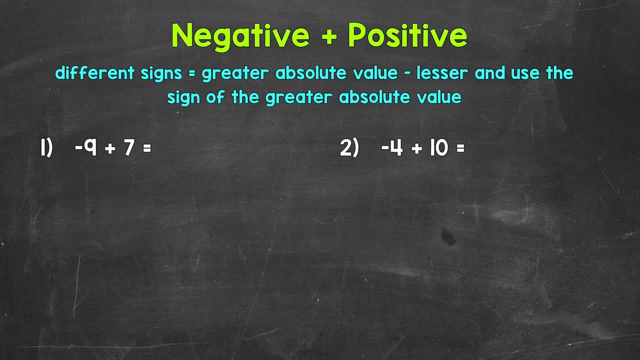 we will take the greater absolute value and subtract the lesser. Our answer will take the sign and subtract the lesser. So we have a negative and a positive. So we have a negative of the greater absolute value. Let's start by rewriting this problem with the absolute values. 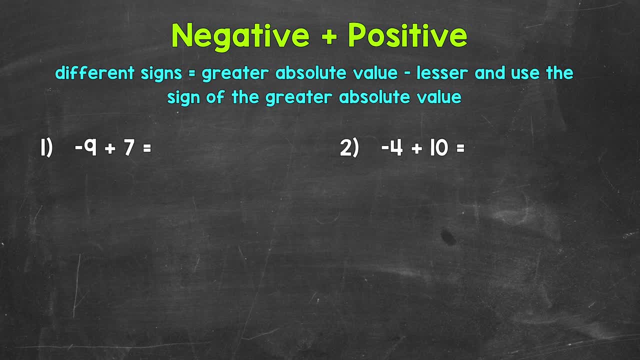 of both negative nine and seven. Now remember, absolute value is the distance a number is from zero. The absolute value of negative nine is nine and then the absolute value of seven is seven. Now we can subtract, So we take the greater absolute value and subtract the lesser, So we take the greater absolute value of negative. 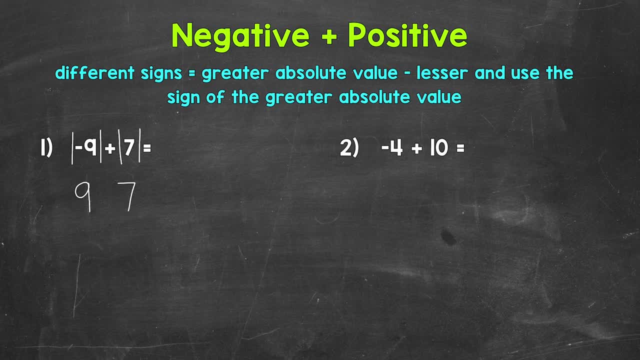 nine and seven and subtract the lesser. These are already in order, so we can subtract If the greater absolute value comes second. we can always switch the order to find the difference, if need be. So we do nine minus seven. That's going to give us two. Now the answer takes the sign of 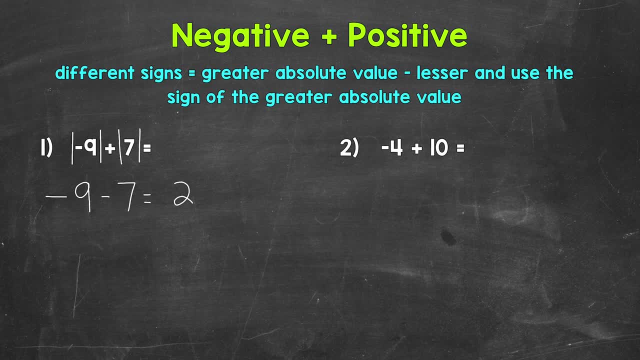 the greater absolute value, The greater absolute value is nine And nine was negative in the original problem, so our answer is negative. Final answer: negative two. Basically, we forgot about any negatives because we were working with absolute values. We found the difference between the absolute values and we took the sign of the greater absolute value. 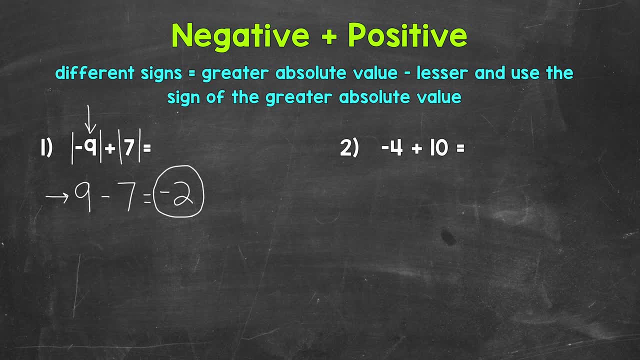 from the original problem for our answer. Now let's think through this a second way, And this way is going to be more of a mental math approach, Just basically thinking about what's going on in this problem. I'll rewrite the problem down below. So we have negative nine plus seven. 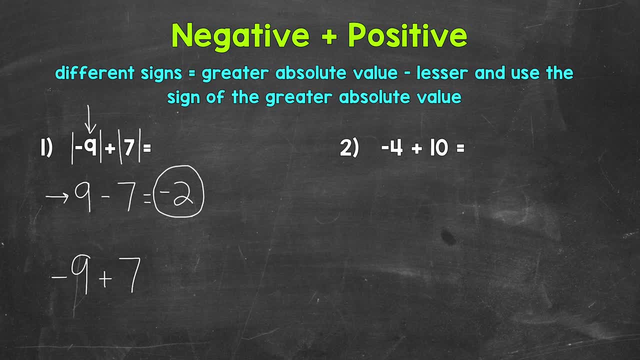 So we are starting at a negative nine and we are adding a positive seven. By adding a positive seven we are increasing in value by seven from that negative nine. Whenever we add a positive we increase in value. So negative nine plus seven equals negative two. So to recap, we started at 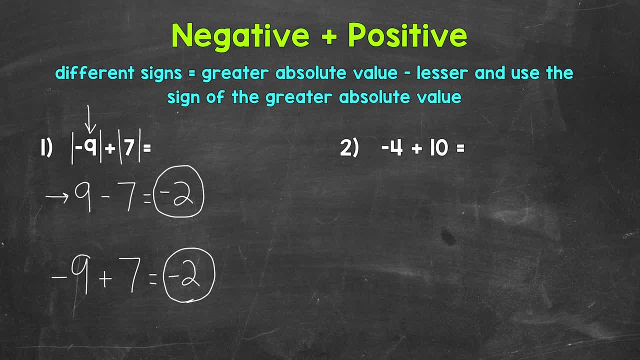 a negative nine. Always think about where you are starting and where you are going from that starting point. So we are adding a positive seven, which is increasing our negative nine in value by seven, and we end up with negative two. Let's move on to number two, where we have 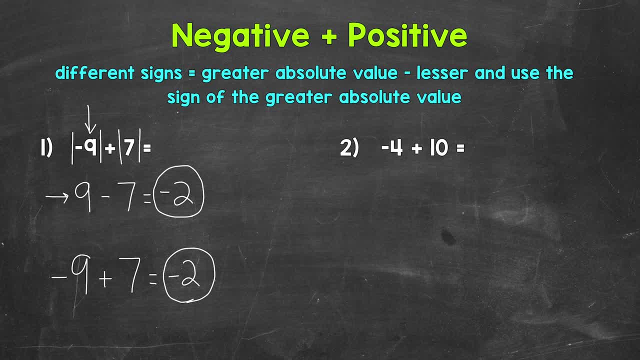 negative four plus ten. So we have a negative and a positive, different signs. Let's take the greater absolute value and subtract the lesser. We'll use the sign of the greater absolute value for our final answer. So let's start with the absolute value of negative four, which is four. 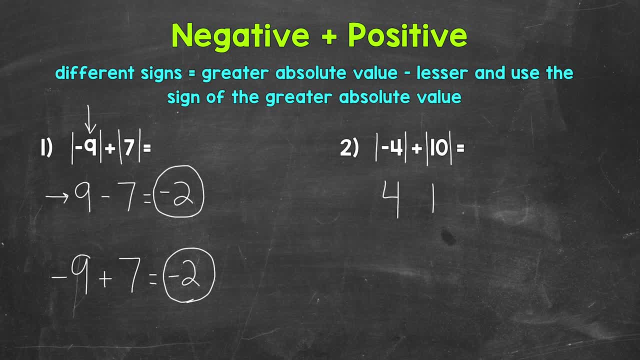 And then the absolute value of ten is ten. Now we need to take the greater absolute value and subtract the lesser in order to find the difference. So let's switch the order here. So we have the greater minus the lesser, so ten minus four, and that gives us six. 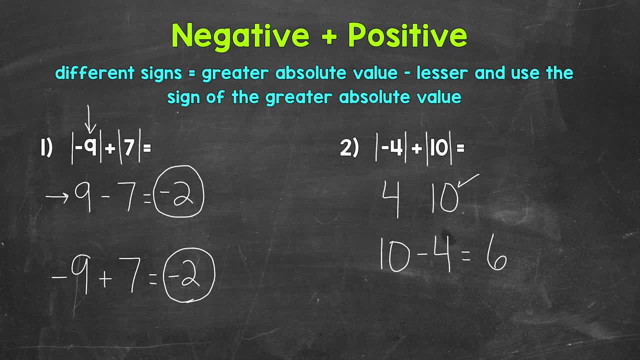 The greater absolute value is ten, and ten is positive in our original problem. so our answer is negative, So our answer is a positive six. Now let's think through this problem. So we have negative four plus ten. So our starting point, so to speak, is negative four and we are adding a positive ten. 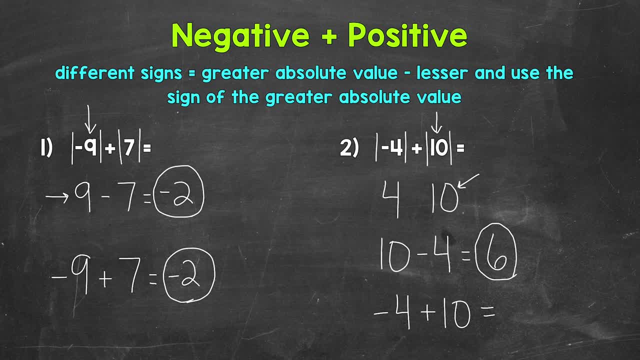 So we are increasing in value. So if we start at negative four and add a positive four, we end up at zero. But we have six more left over from that positive ten and we end up at a positive six. So starting point: negative four. add that positive ten, we end up at a positive six.